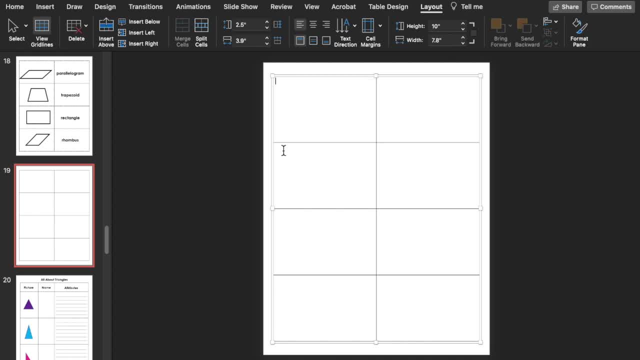 the back of the shape. Be creative with these flashcards featuring two-dimensional shapes To get our shape in our cells. we're going to go to insert and go over to shapes and we're going to focus on quadrilaterals. I'm going to start with a rectangle. 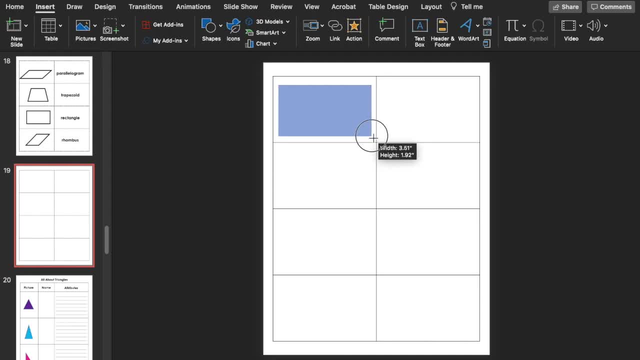 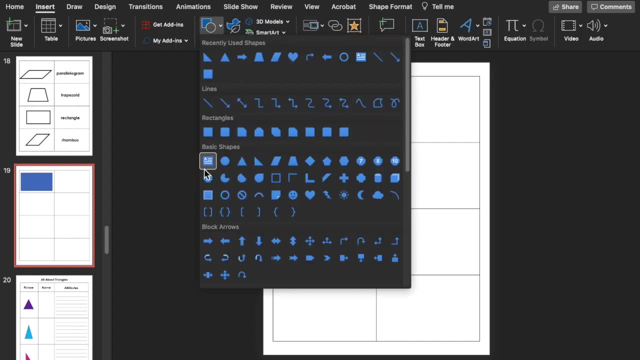 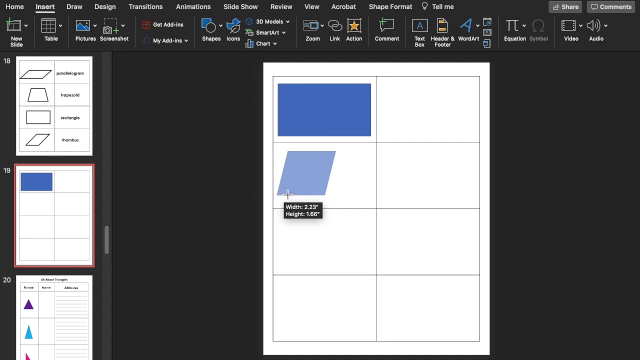 and create that rectangle here and let go. I'm going to go back to insert and go back to shapes. We're going to do a rhombus next. This is going to pre-prequelle it and I'm going to go back to shapes and it's going to go to: 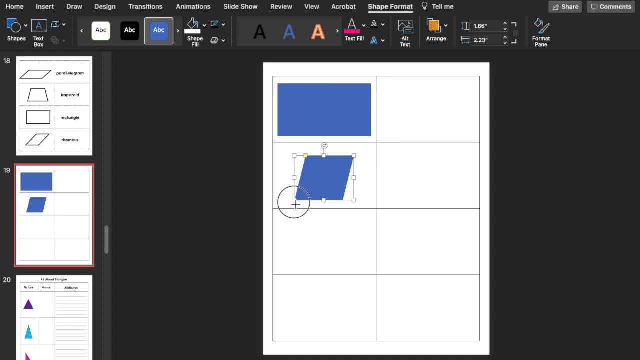 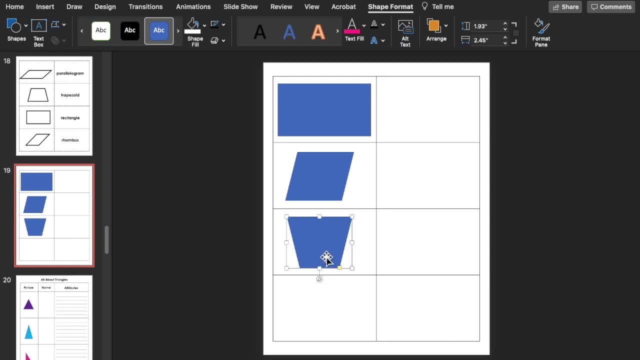 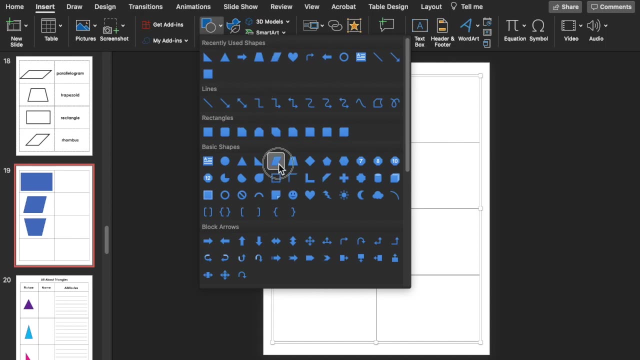 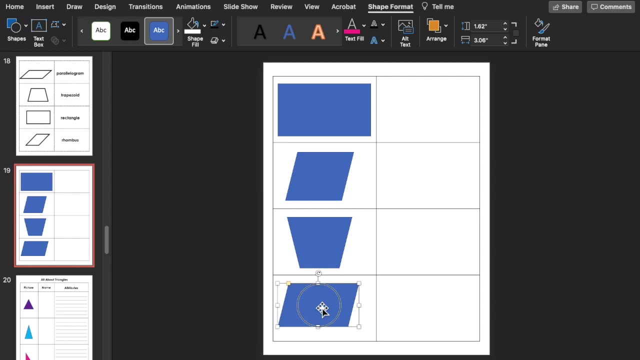 that you want, and then we're going to repeat that rhombus, but extend the sides, the top and bottom, so that it's just a parallelogram and not a rhombus. I want to change the color. I'm going to select all the shapes. I did that by holding the command. 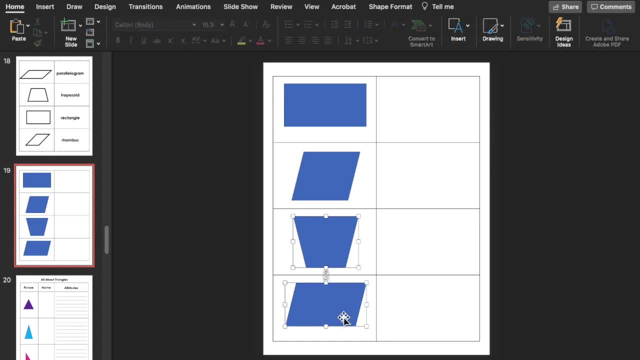 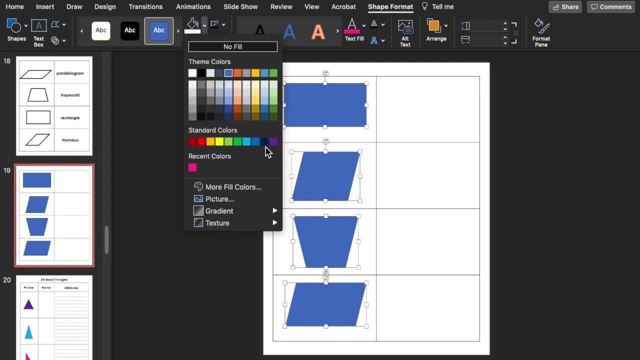 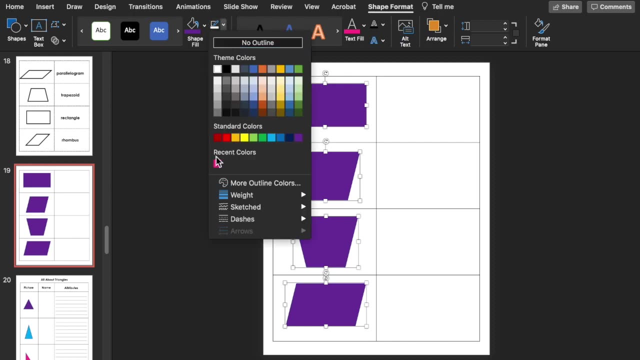 key down and then clicking on the shapes which selects them or deselect them. so now I'm going to go up to shape format, go over to shape fill so you can give it a specific color and a specific outline, if you want. or we can make a black and white copy so we have a white fill with a black line and then I'm going. 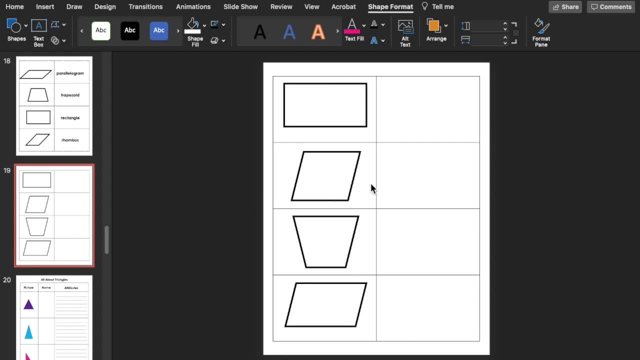 to make the weight of the line four and a half. so there are our shapes, our 2d shapes, quadrilateral specifically. so now I'm going to go to insert a text box to write the names of each of the shapes. so we have a rectangle. duplicate that by hitting command d or control d if you have a pc, and we have a bombus. 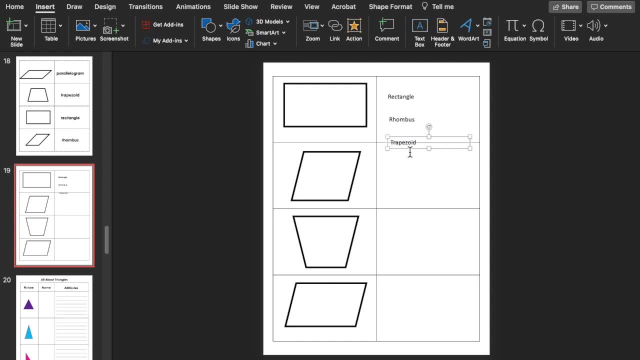 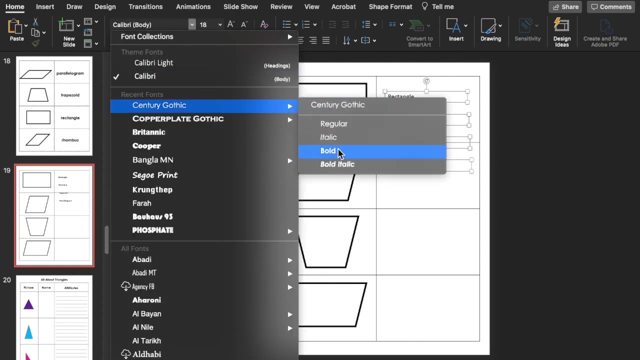 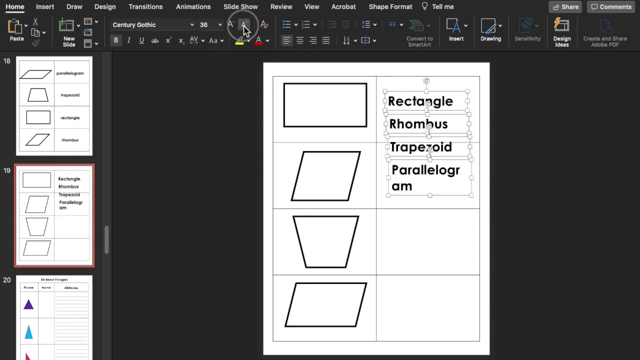 and we have a trapezoid and a parallelo. so now I'm going to select each of the text boxes and we're going to change the size and the font with them to all fit on one line. we're going to center them and there we go. so here's our parallelogram. 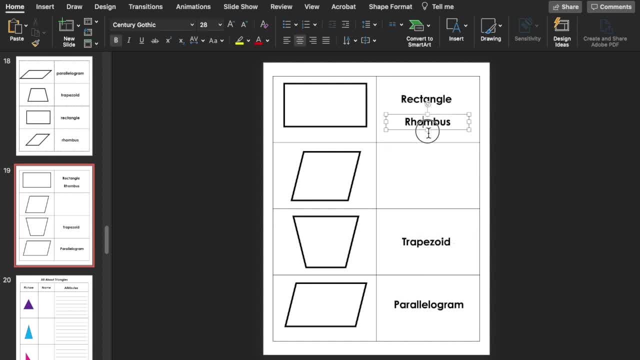 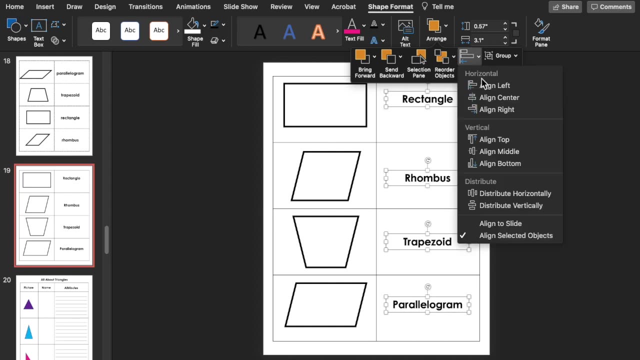 and i'm just going to bring this down here and then this one down here. i'm just going to select these all so i can line them up. so i go to shape format, arrange, align center, and then i'm going to go to align, distribute vertically so that they're all equally distributed. 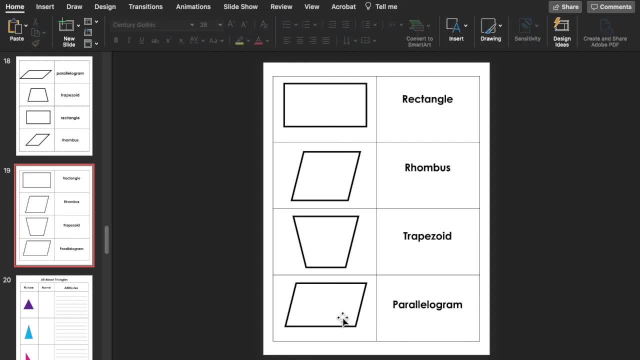 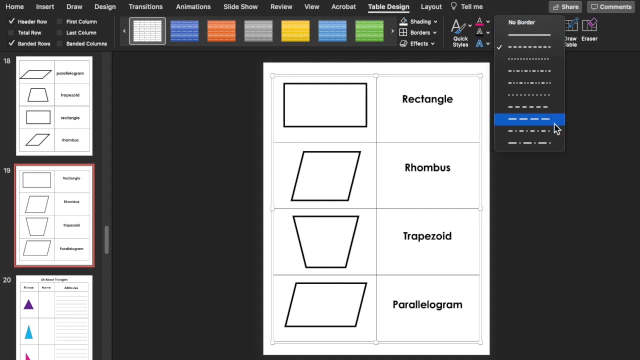 all right. so there are our two-dimensional shapes, as well as their words, and then the last thing i'm going to do is change the line to be like that dash or dotted line. so i selected the table, i'm going to table design and then i'm going to select the type of line i want on the border. 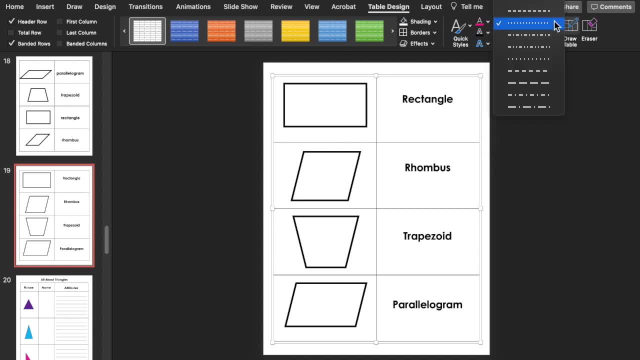 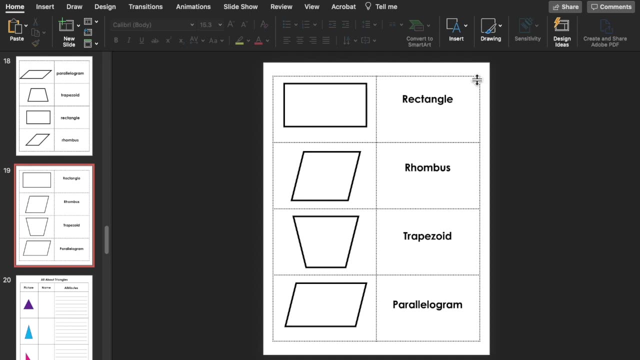 so i'm going to go with this first one. actually, the second one, more of a dotted dash, make sure my pen color is black. and then i'm going to go to borders and select all borders and there's that dotted line students can cut on. i think i do want to change it to that first dash. 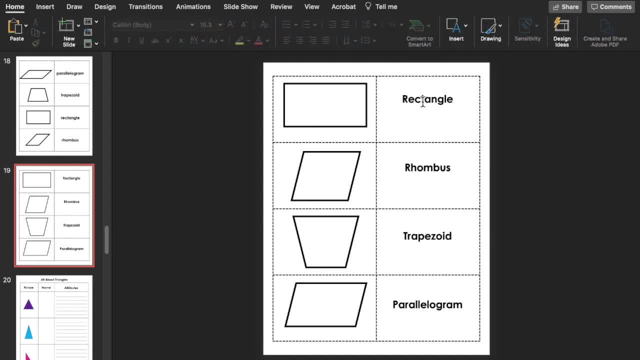 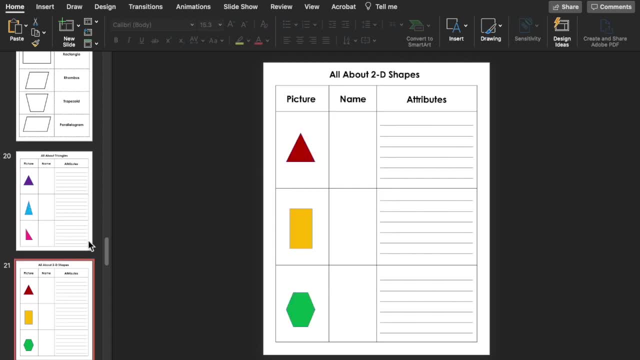 i like that one a little bit better, so they definitely know that we want them to cut these out. so the next type of examples are kind of like a note sheet that students can take as they're learning about the different triangles or different two-dimensional shapes. whatever focus that you have for your shapes we're going to create. 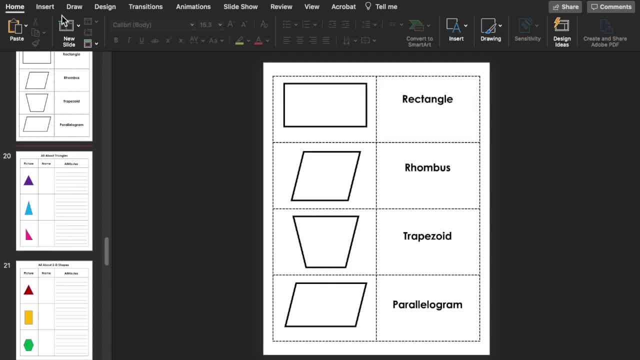 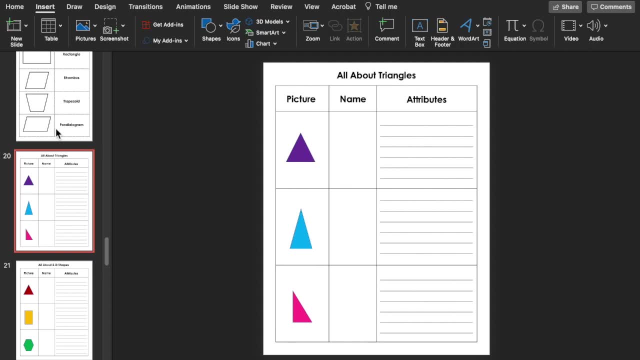 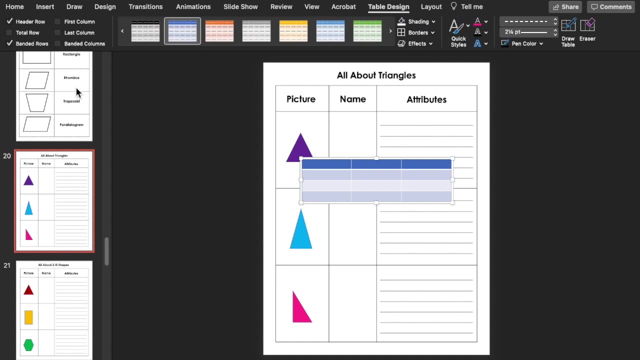 like a notes page. so we're going to insert a new table and we want it to have three columns and four rows in each column. go back, let me insert that blank page and then i'm going to go back and insert that blank page. let me insert that blank page and then i'm going to go back and insert that blank page. 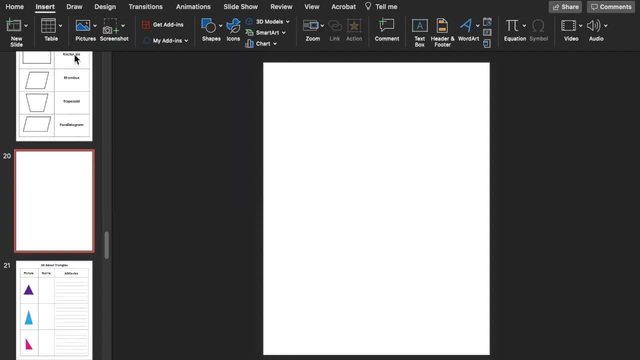 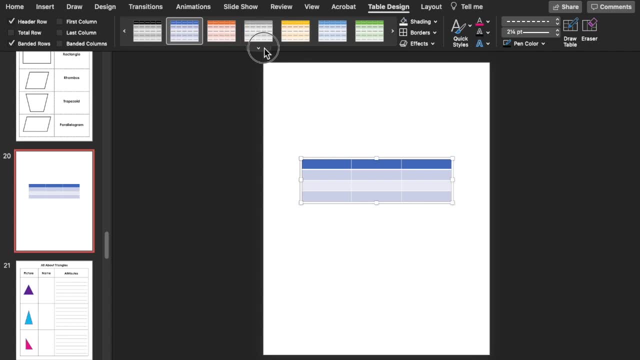 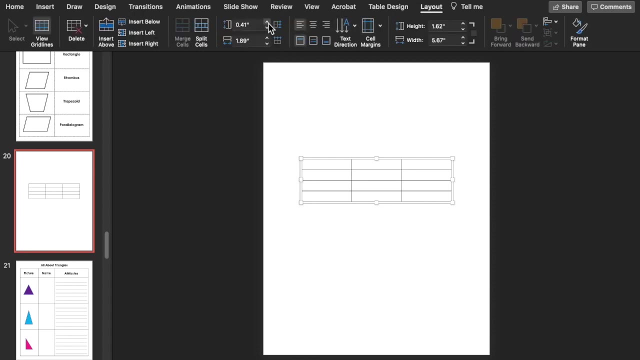 again, here we go: insert table three columns with four rooms. we're gonna go to the table design, click on no style and then go to layout and then increase and we're gonna bring this up. i do want to leave space for like a title, and i'm actually going to. 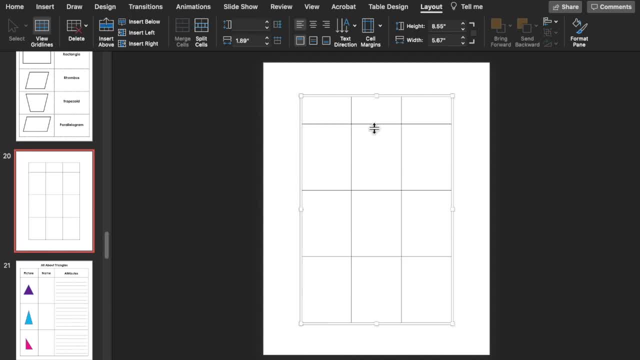 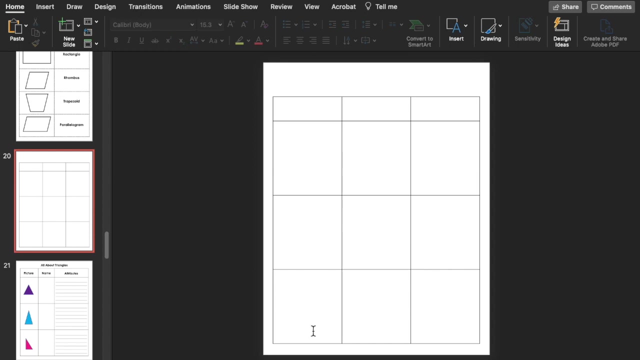 make this first row a little bit smaller, because that's where we're going to put our labels. but everything else can be stretched out a tad bit more, and then we are going to extend the width of the cells. that's perfect. we're going to have a column for picture, column for the name. 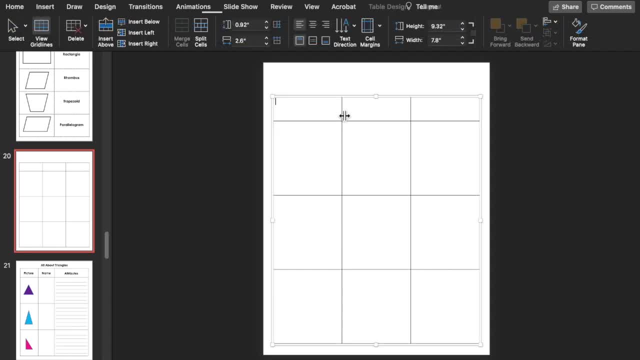 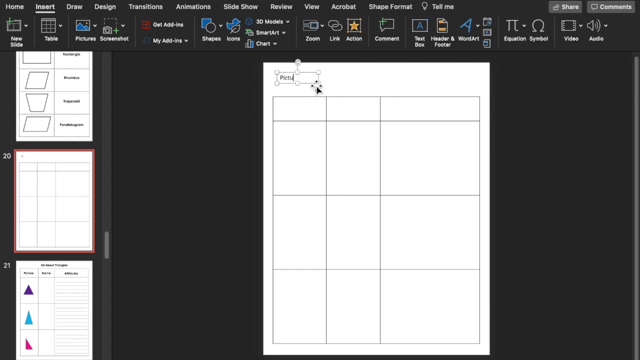 and then a column for the attributes. so we're going to have a column for picture, column for the name and then a column for the attributes. so i do want attributes, so i do want attributes. so i do want the picture. the picture, Select it, go to home center. it make sure it's in the middle of the box, change the. 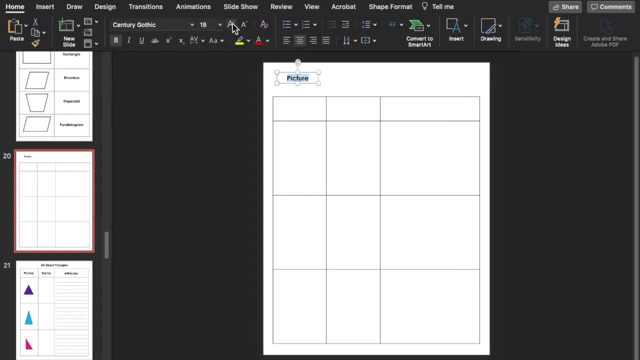 font and increase the size. that looks good And I'm going to select it and duplicate it again. command D on your keyboard or control D if you have a PC. I'm going to change this to name. I'm going to hit duplicate again. 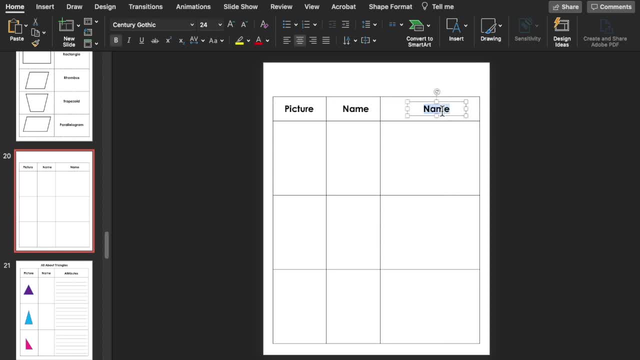 stretch this out and change this to attributes, or some people like to put characteristics, Alright, so now we're going to add in- oh, let's add in one more text box for our title. I'm going to call this all about triangles. 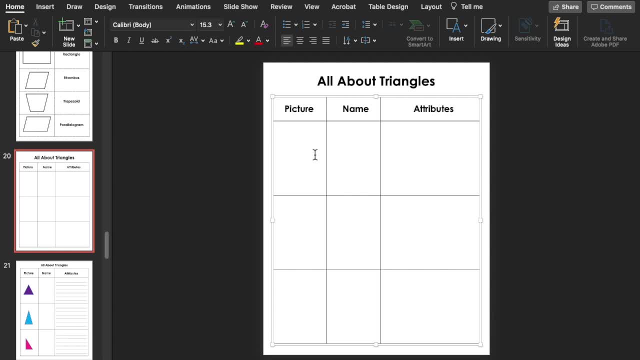 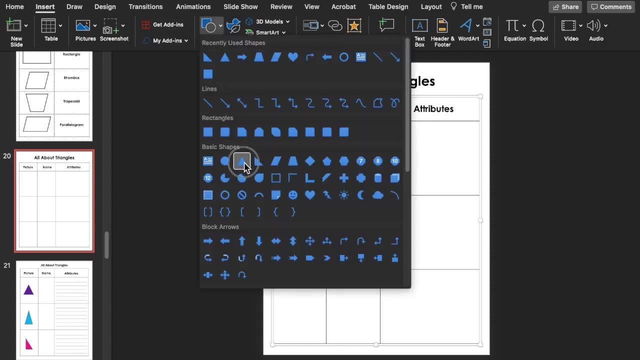 So you can always do multiple pages to do, categorize triangles by their side length or you can organize them by their angles. So we're just going to focus on sides. So I'm going to go to the top page, go to insert and choose some triangles that they have. I'm gonna go to this. 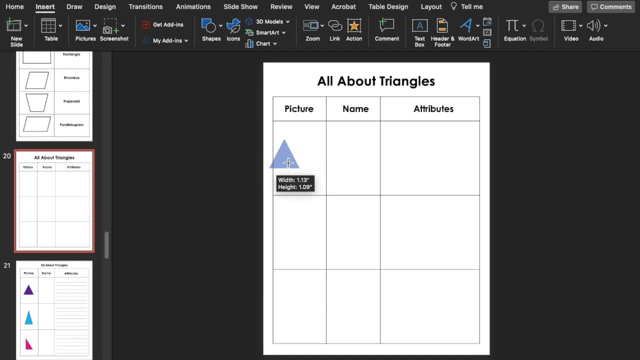 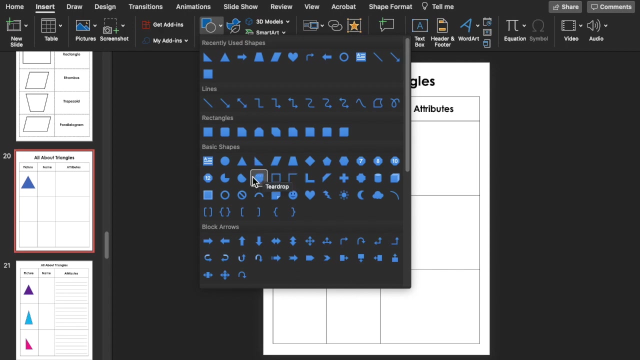 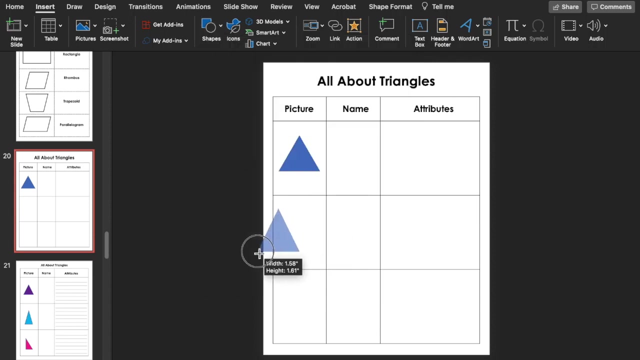 triangle and make like an equilateral triangle where all the sides are the same. then I'm going to go back to insert shapes so those three sides are the same. so I'm looking for another triangle. or I'm going to create another triangle where the sides are not the same. so the same triangle, but I'm gonna make the two. 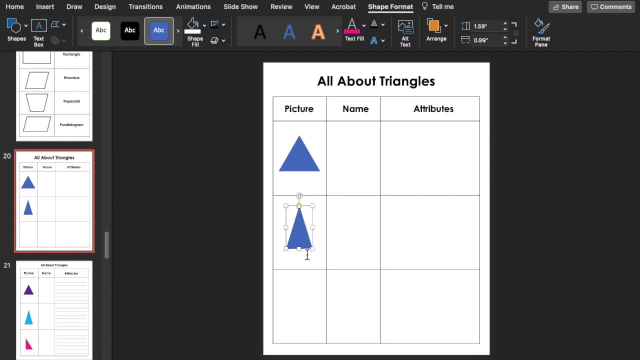 sides here the same and in the bottom one is different. so represent I saw- Sully's triangle and then we're going to go back and insert one more time. you can also duplicate the triangles if you want right triangle and make sure that the sides are all different. to represent a scaly triangle: 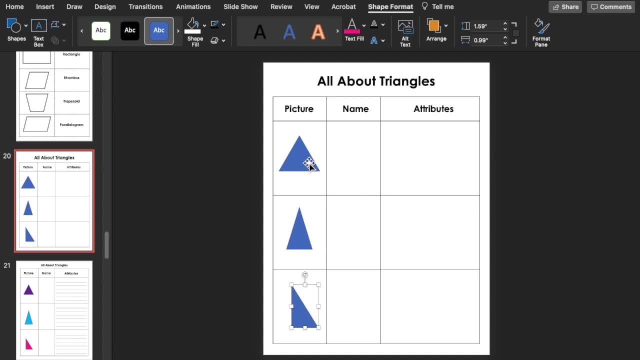 where none of the sides have the same length and you can leave it blue. you can change these to colored triangles or you can make them a black line, where they have a white fill and just a black outline, and then thicken that the weight of the line. so those are your options. be creative with your. 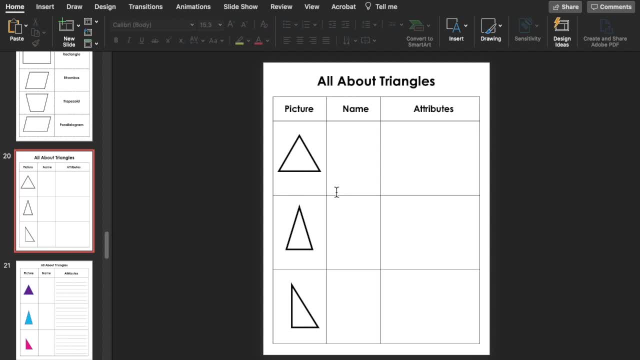 you printables, and it all depends on what kind of ink you have with your printer. you have access to a color printer, then great. so then we're going to leave the spot for name blank. but for attributes you can leave it blank and have them right freehand, or you can add lines if you like. so I'm going to insert another. 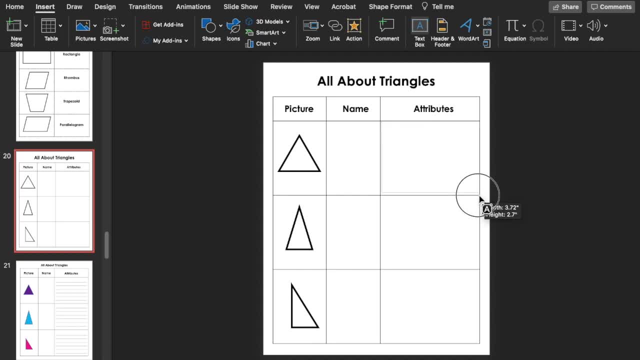 text box and I wanted to stretch the size of the cell, and then I'm going to hold this shift key down on my keyboard and then press on the dash button on the keyboard and just spread it out all the way down the cell. ok, ok. so there is your text box with lines. now I'm going to do it again. start to sign. with one oubliette: again you have to tick dejected. if a textbox is full or the doesn't indicate the number on your screen, you can use the alt key to exit and press gallery keys, or hit Hut or Alt key to exit. 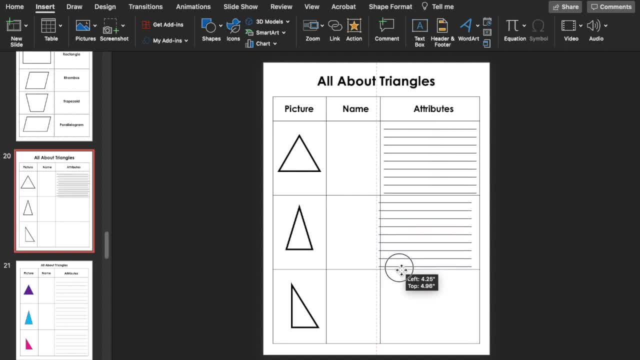 duplicate this, place it down here in the second box and then duplicate it again. now, if these lines are too small for your students, you want to give them more space. something you can do is get rid of the bottom section of lines, and then, if you select them all again and go back to the home tab, you find your button that.